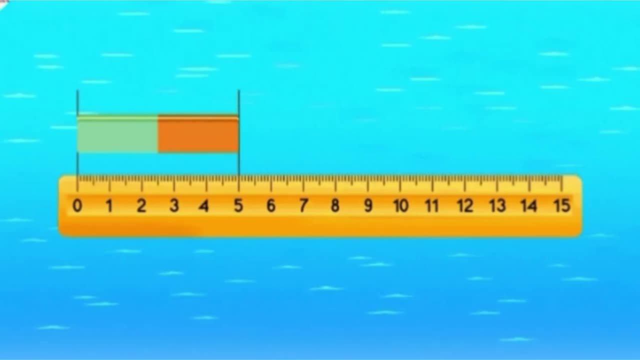 Pay attention to the other end of the eraser to get the result. The eraser is five centimeters long. Let's use another example. How long is the crayon? Well, the crayon is seven centimeters long. What about the pencil? 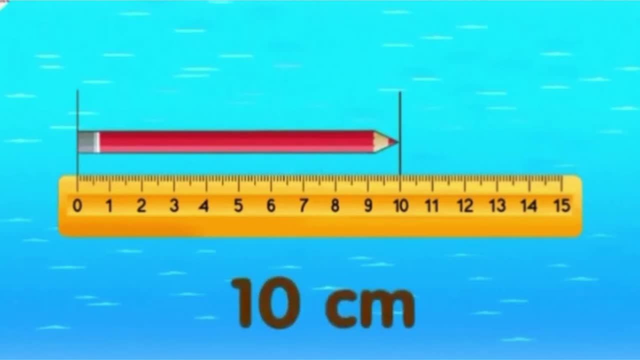 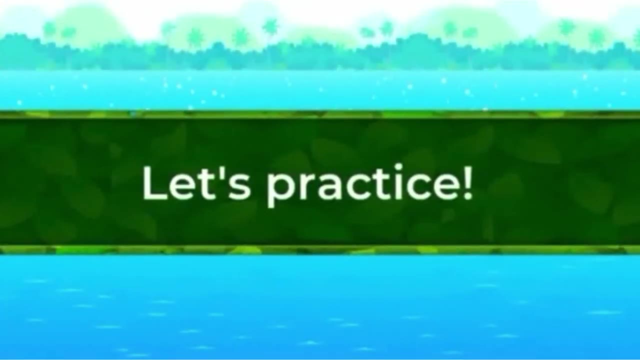 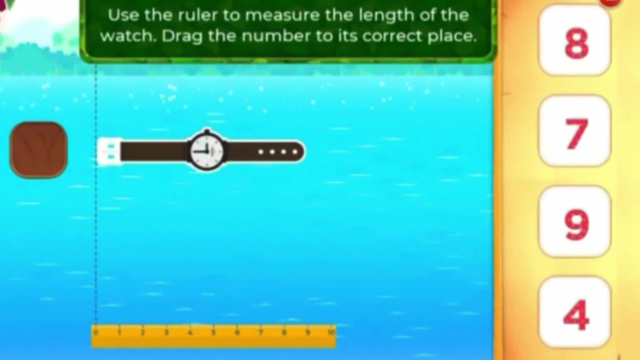 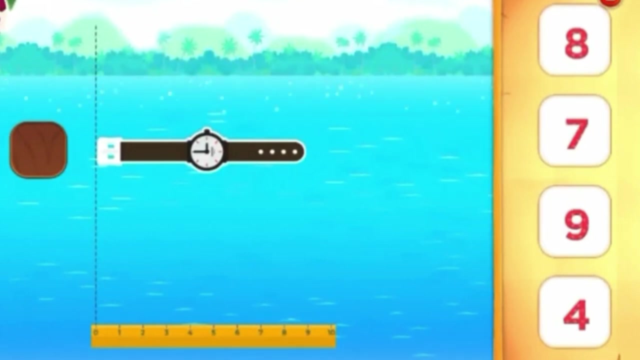 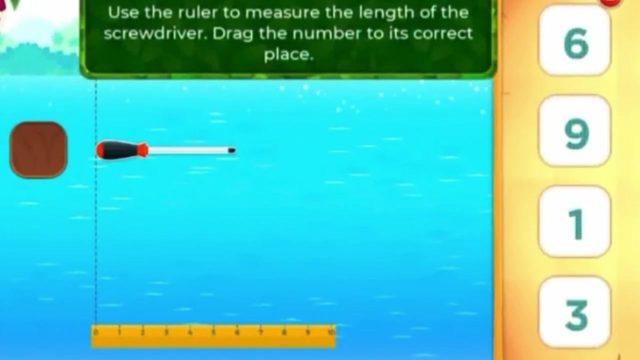 The pencil is ten centimeters long. Get ready, Let's practice now. Use the ruler to measure the length of the watch. Drag the number to its correct place. You did it. Use the ruler to measure the length of the screwdriver. 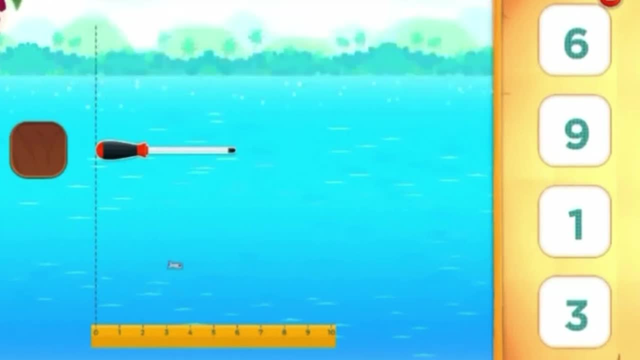 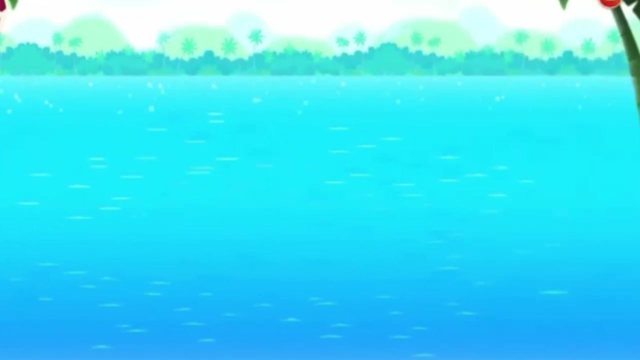 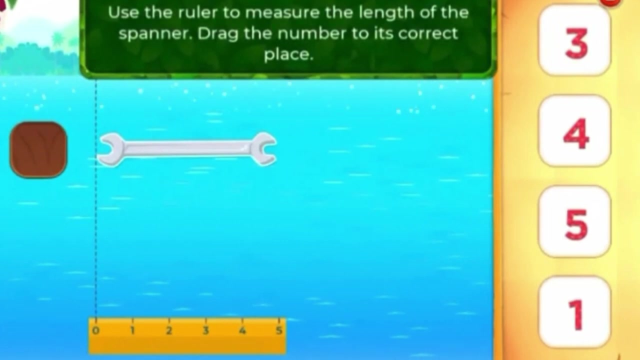 Drag the number to its correct place. You did it. Use the ruler to measure the length of the watch. Drag the number to its correct place. You did it. Use the ruler to measure the length of the watch. Drag the number to its correct place. 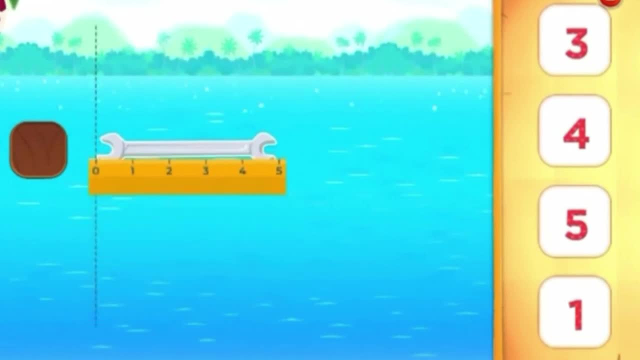 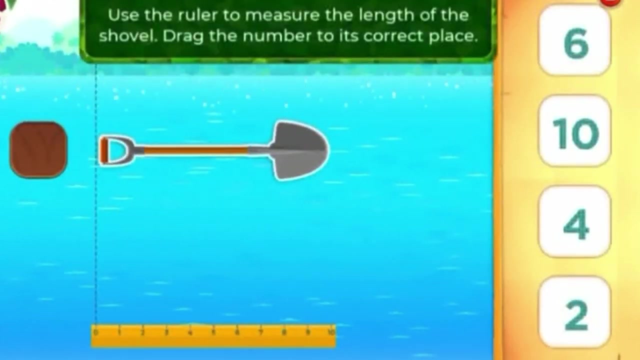 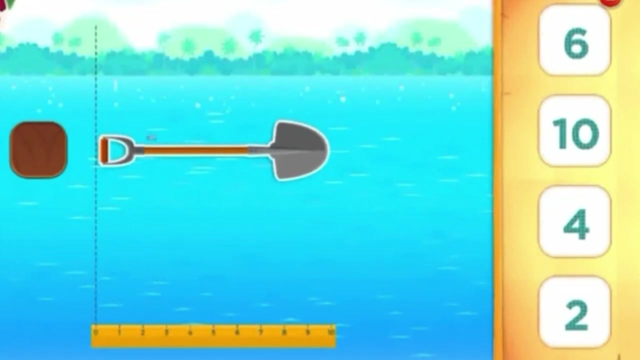 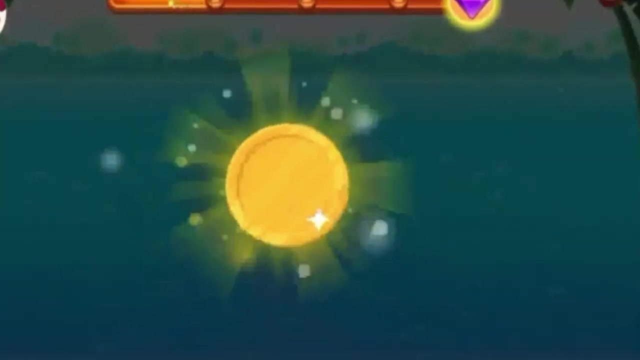 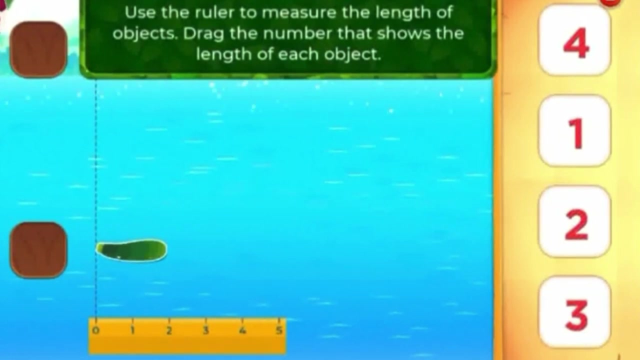 Use the ruler to measure the length of the watch. Drag the number to its correct place. Drag the number to its correct place. Use the ruler to measure the length of the watch- Good job. Use the ruler to measure the length of objects. Drag the number that shows the length of each object. 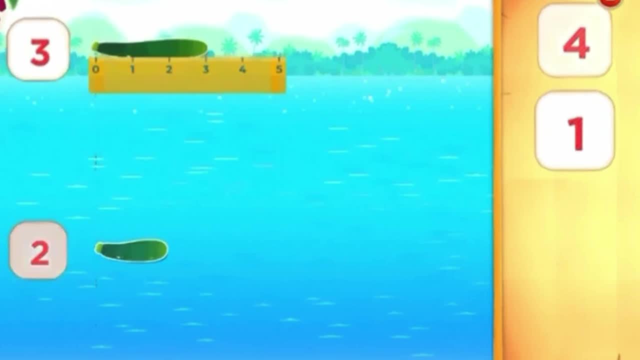 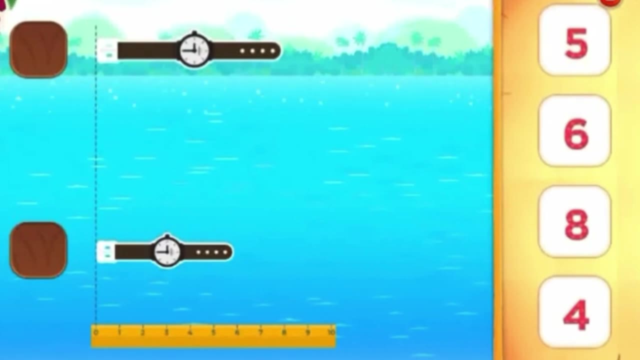 Use the ruler to measure the length of objects. Drag the number that shows the length of each object. Use the ruler to measure the length of objects. Use the ruler to measure the length of objects. Drag the number that shows the length of each object. 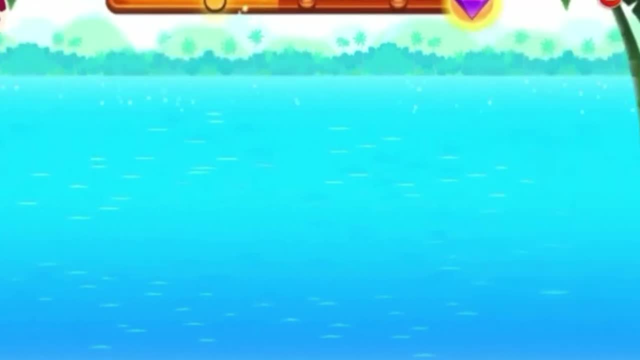 Use the ruler to measure the length of objects. Use the ruler to measure the length of objects. Use the ruler to measure the length of objects. Drag the number that shows the length of each object. Use the ruler to measure the length of objects. 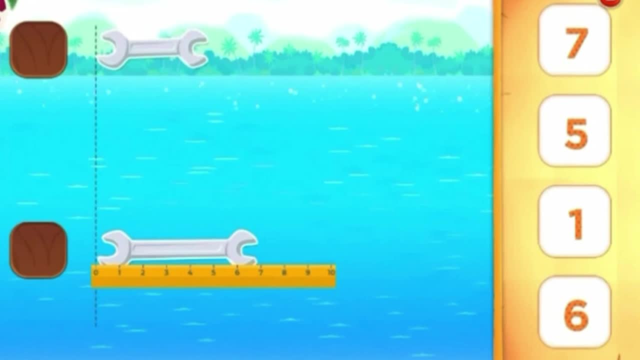 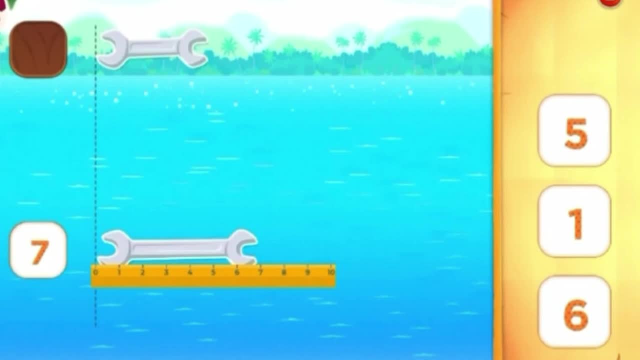 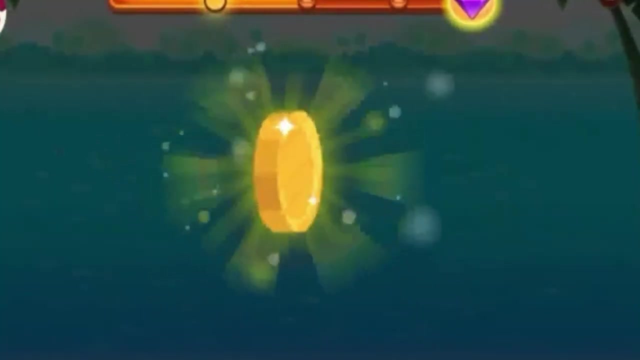 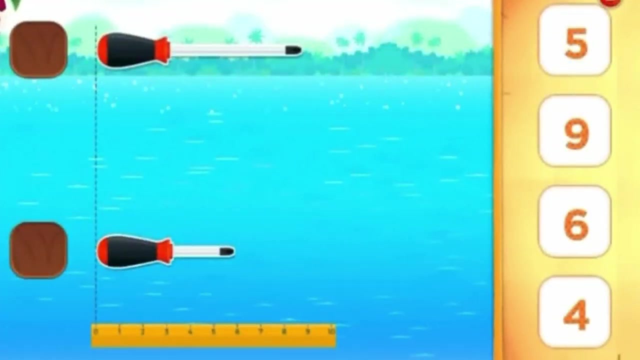 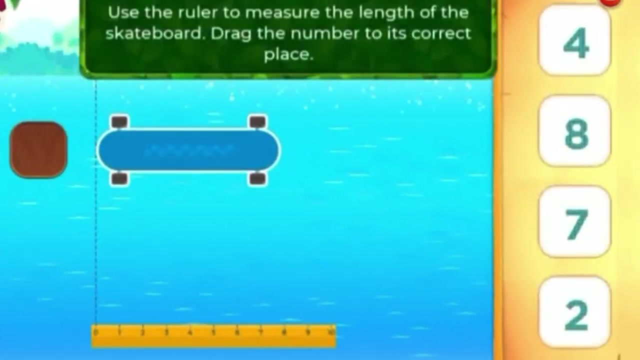